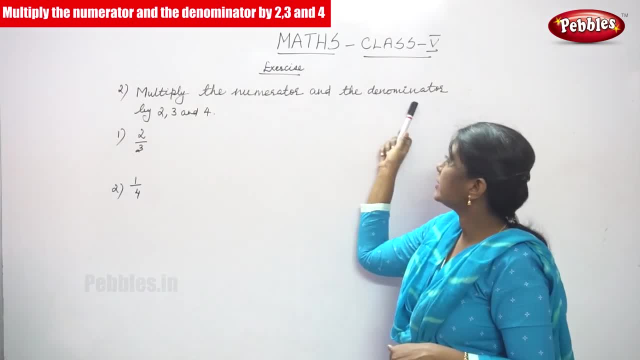 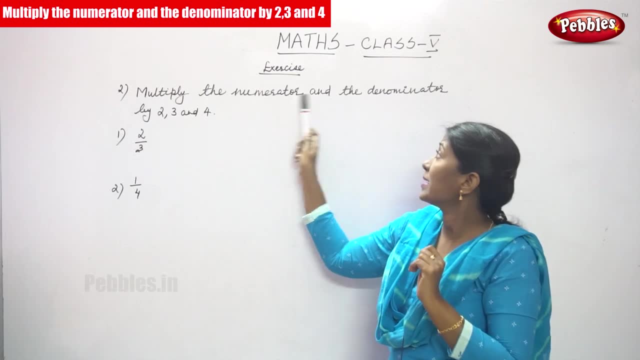 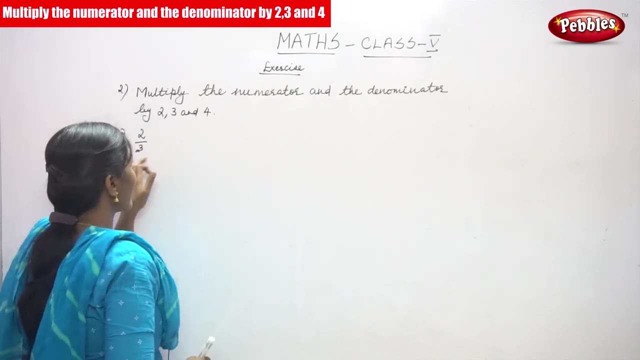 Next suggestion is: multiply the numerator and the denominator by 2,, 3 and 4.. So multiply the denominator. sorry, multiply the numerator and the denominator by 2,, 3 and 4.. So this is the fraction is given, So this fraction is multiplied by 2, 3 and 4.. So first you have to multiply with. 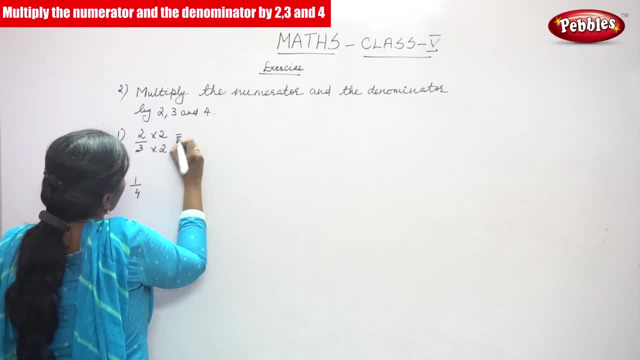 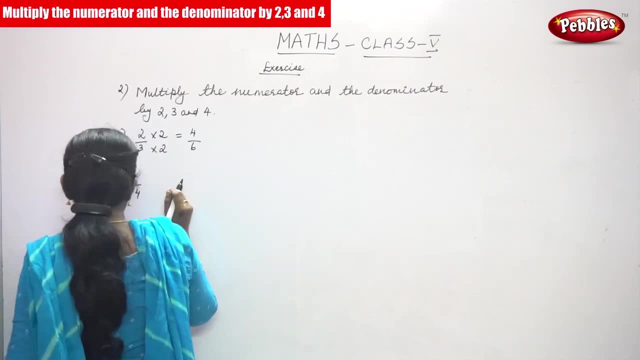 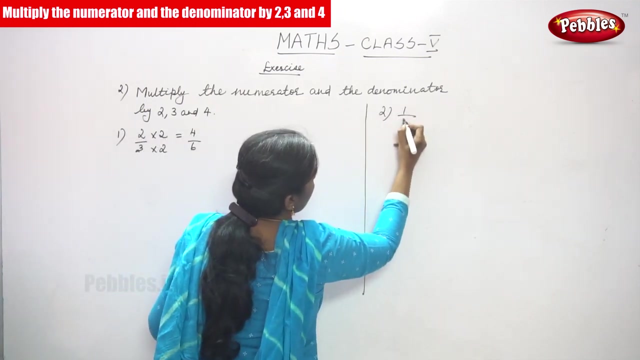 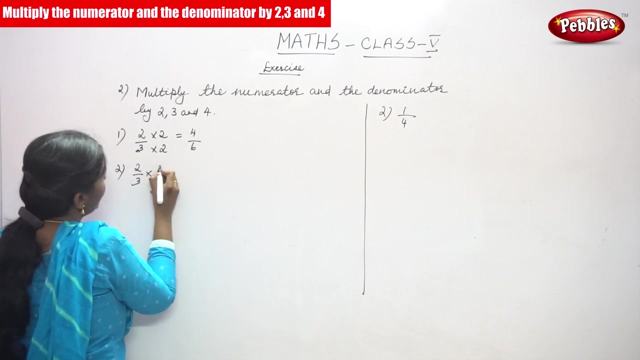 2.. What is the answer? 2 into 2,, 4,, 4 by 6.. Next again, you will get what. So next is what It is: 2 by 3 is multiplied by 3.. The numerator and the denominator is: 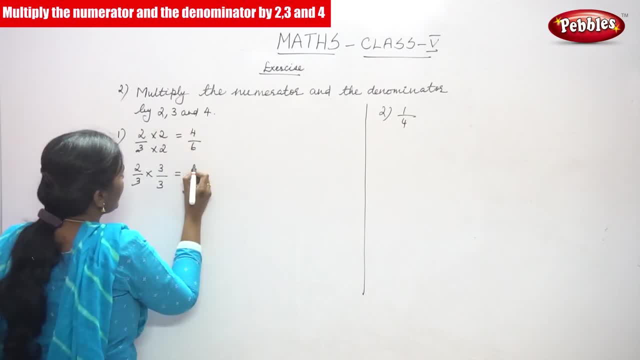 multiplied by 3, because 2 into 2, 4, 4 by 6.. So next again you will get what It is: 2 into 2, 4, 4 by 6.. So next in this question is given 2 into 3, 6.. 3 into 3, 9.. Next, 2 by 3 into 4 by 4.. So 2 into 4, 8 and 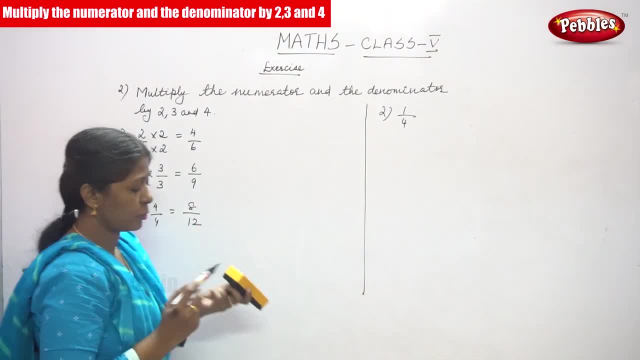 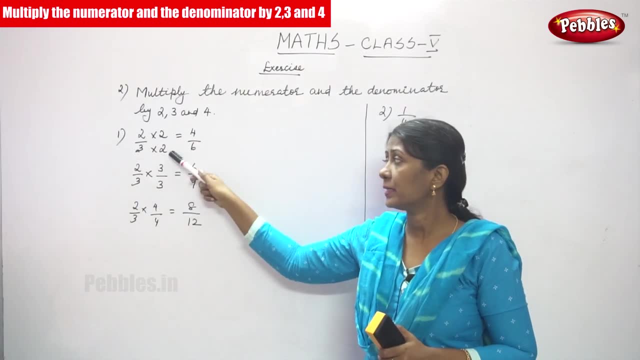 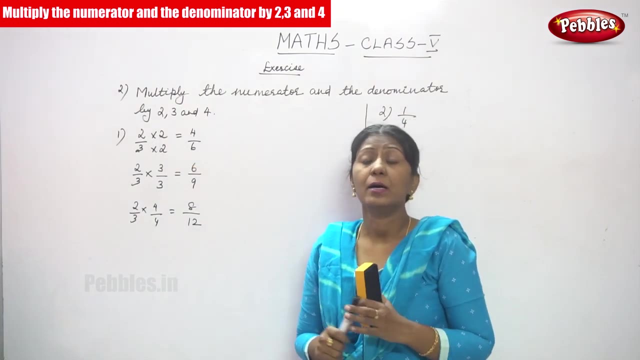 3 into 4, 12.. So first you have to, first you have to multiply 2 by 3 into 2, then 2 by 3 into 3,, 2 by 3 into 4.. So 2 by 3 into 2.. The multiply, multiply, the multiply, the numerator and the 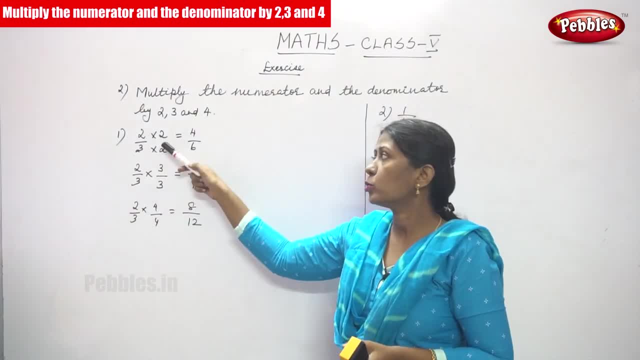 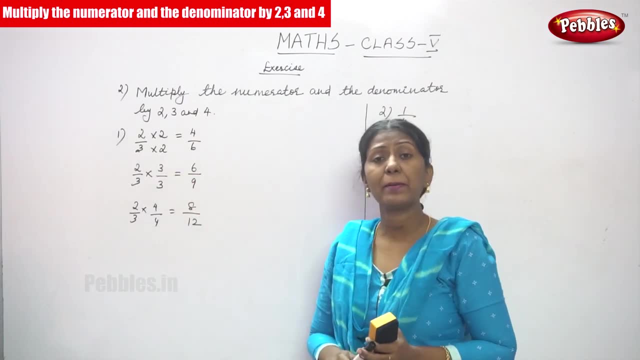 denominator by 2.. So 2 by 3 is multiplied by 2.. So 2 into 2, you can get 4.. 3 into 2, you can get 6.. Next, the same 2 by 3 is multiplied by 3.. The numerator and the denominator, both number is: 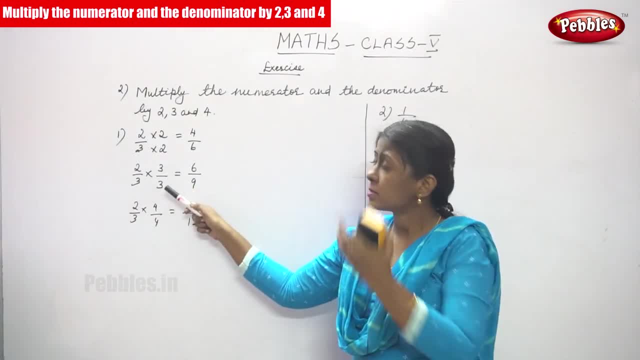 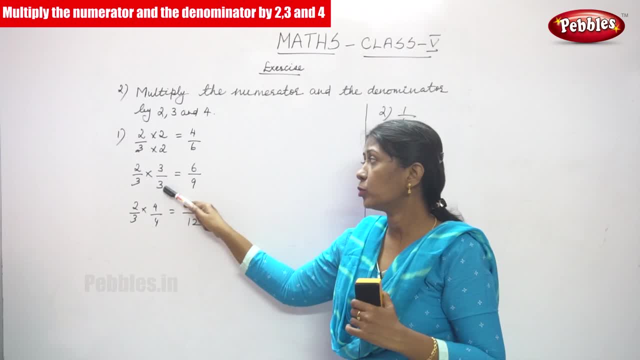 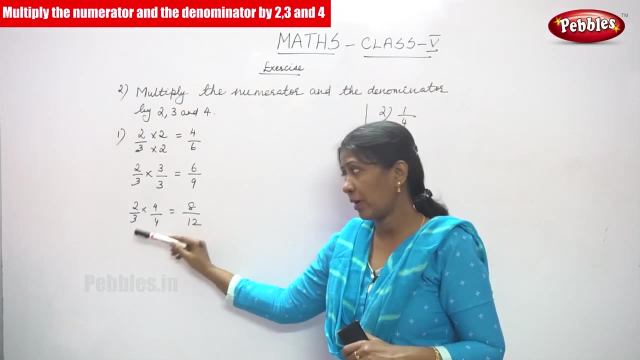 3. so 2 into 3 you can get 6, and 3 into 3 you can get 9. so next is: 2 by 3 is multiplied by 4, so the numerator is multiplied by 4 and the denominator is multiplied by 4. that is the. 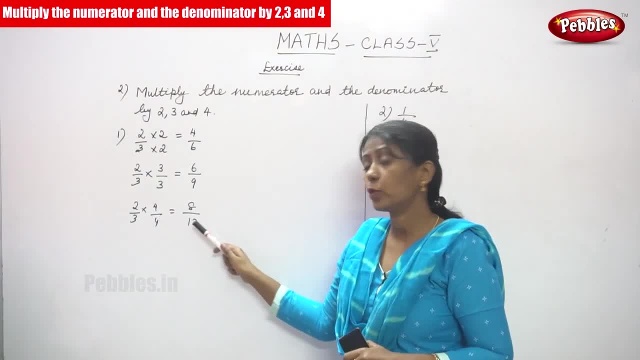 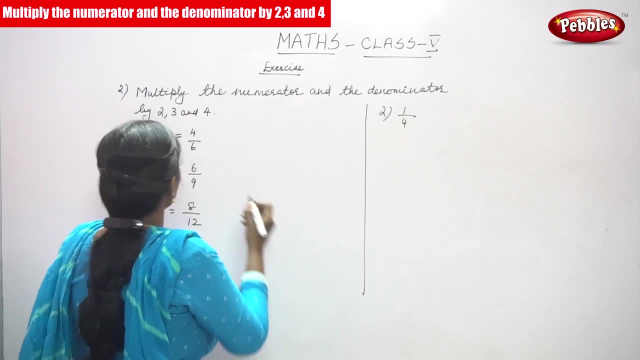 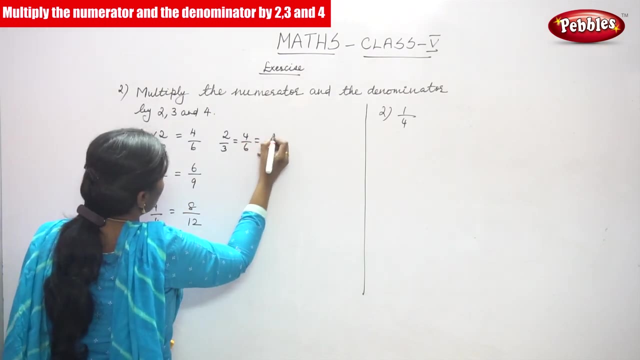 rules. so 2 into 4, you can get 8, and 3 into 4, you can get what 12? the answer is: 4 by 6, 6 by 9, 8 by 12. so have to write it: 2 by 3 is equal to what? 4 by 6 is equal to 6 by 9 is equal to 8 by 12. so 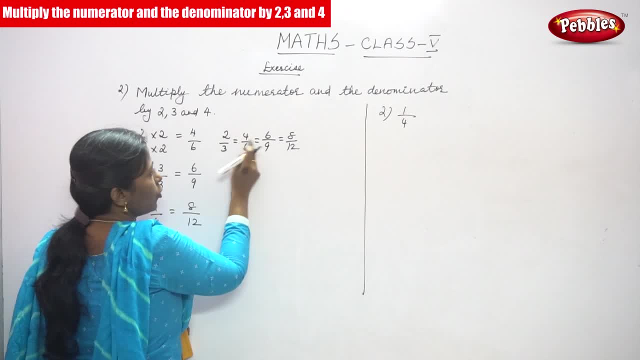 these are the equivalent fraction again, so 2, 4, 6, 8, 3, 6, 9, 12. so this number is multiplied by 2, you can get 4 by 6. again 2 by 3 is multiplied by 3, you can get 6 by 9. so again 2 by 3 is multiplied. 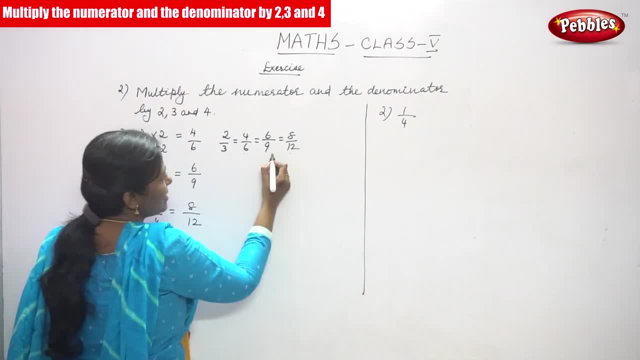 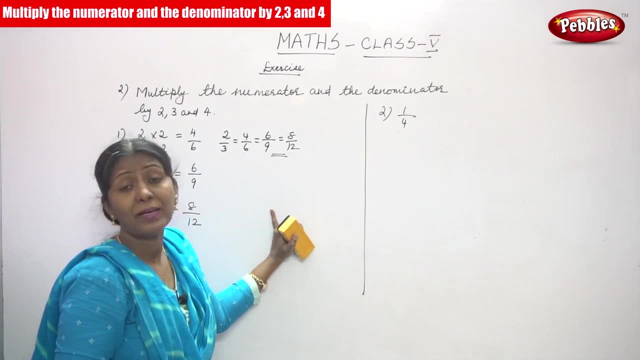 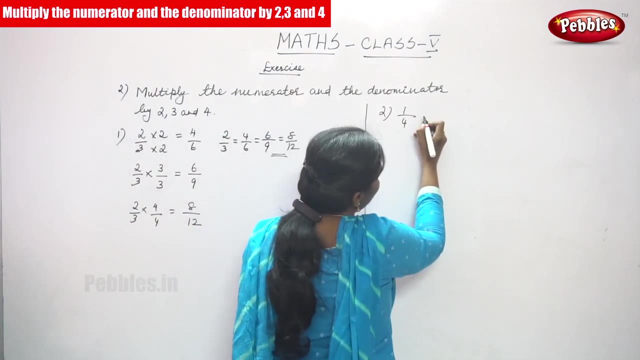 by 4, you can get 8 by 9, 8 by 12.. So this is the. this is the answer for this question. So you can find what you can find: the equivalent fraction, but different multiples. we are using here The same. one more sum is 1 by 4.. So 1 by 4 is going to multiply by 2 first. So the numerator and the 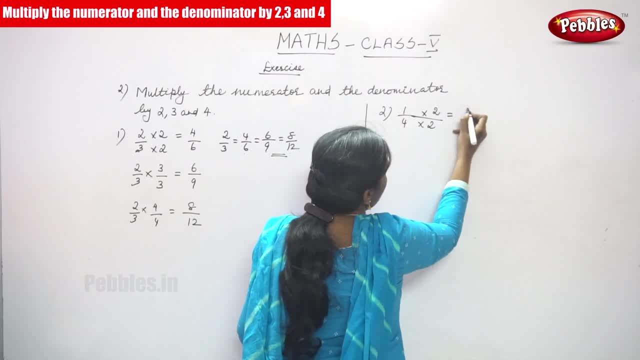 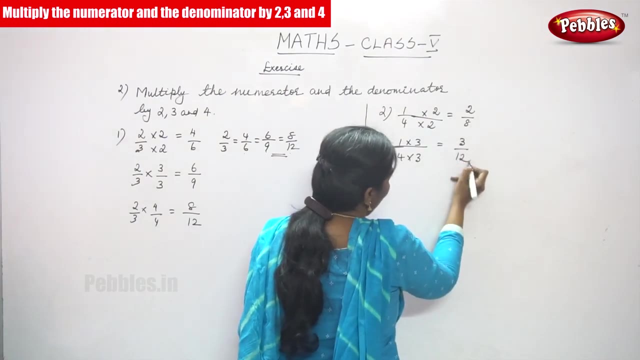 denominator. both number is multiplied by 2. The answer is: 1 into 2 is equal to 2.. 4 into 2, you can get 8.. Next again, 1 by 4 is multiplied by 3. So answer is: 1 into 3, 3. 4 into 3, 12. Next, 1 by 4. 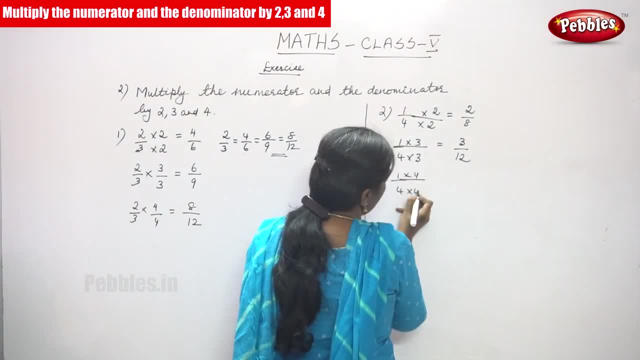 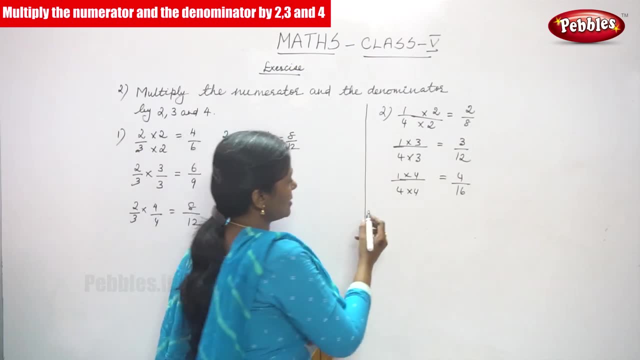 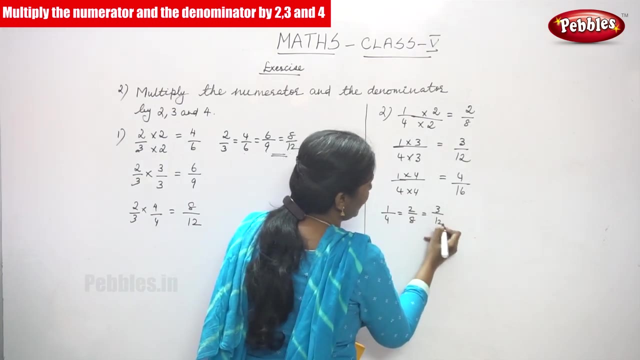 is multiplied by 4.. So 1 into 4, you can get 4.. 4 into 4, you can get 16.. So what is the answer? So 1 by 4 is equal to 2 by 8 is equal to 3 by 12.. 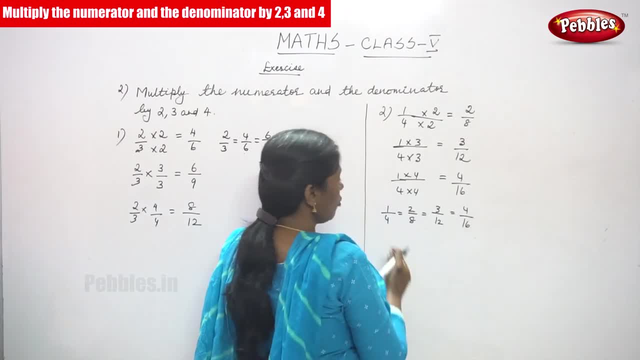 Is equal to 4 by 16. So first, 1 by 4 is multiplied by 2. So you can get 2 by 8. Next, the same 1 by 4 is multiplied by 3. You can get 3 by 12.. Next, 1 by. for the same 1 by 4 is multiplied by 4. You can.